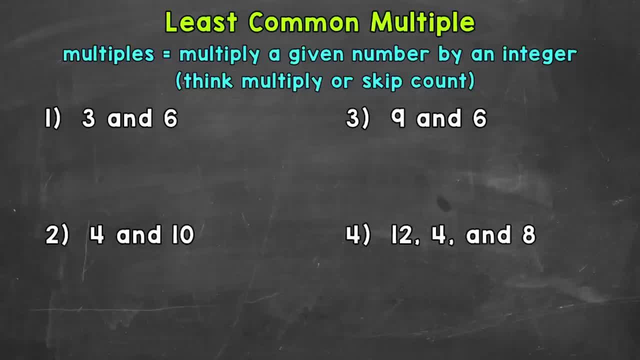 Think, multiply or skip count when you think of multiples. Now, that may sound a little confusing, but it's actually not too bad. I think an example will make it much more clear. So let's jump into number one, Where we have three and six. 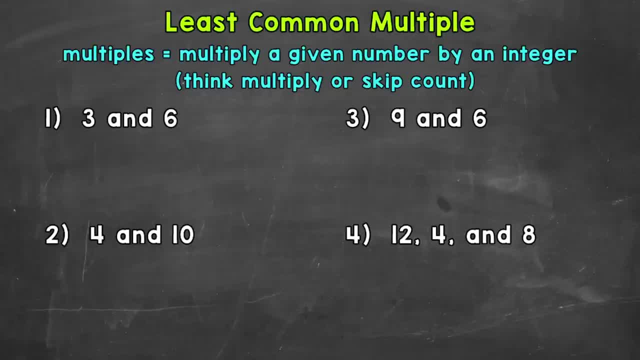 Let's start with some multiples of three And remember: think, multiply or skip count. So let's write the first five multiples of three And then we'll go from there. So three times one is three, Three times two is six, Three times three is nine. 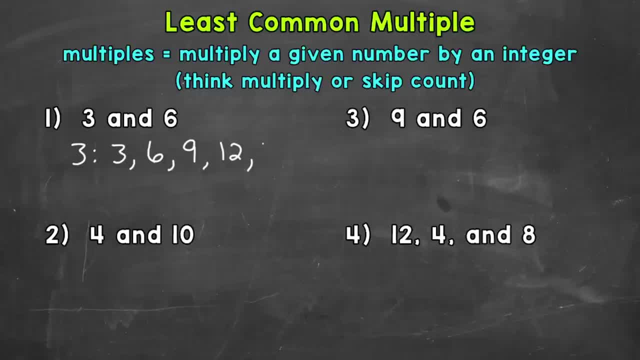 Three times four is twelve. Three times five is fifteen. So I'll stop there And then we'll write some multiples of six and see if we have any in common, And if we do, we're going to look for the least that they have in common. 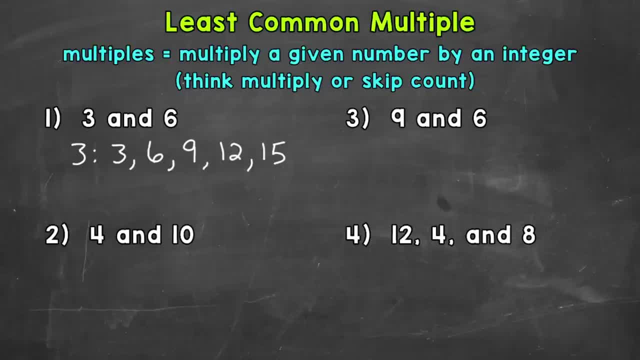 Now those multiples go on forever. So I suggest writing four or five multiples for each given number, See if you have any in common and then go from there. You can always extend your lists of multiples. So let's write some multiples of six. 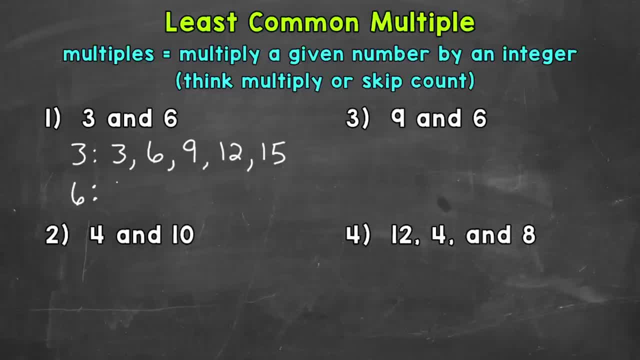 So again, think, multiply or skip count. So six times one is six, Six times two is twelve, Times three is eighteen, Times four is twenty-four, And then times five is thirty. So we did five multiples for each. Let's see if we have any common multiples. 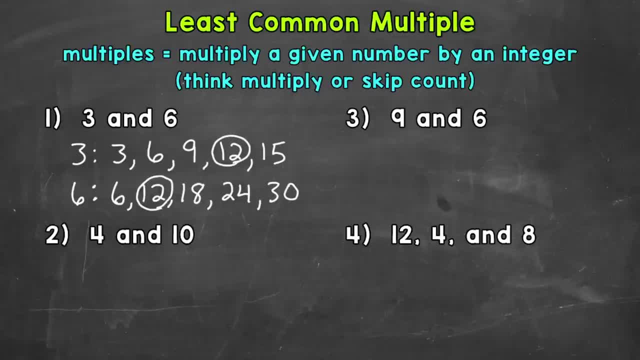 So we have twelve in common And we also have six in common, But we want the least. So six is going to be the least. It's going to be the least common multiple between three and six. So I'll put LCM, which stands for least common multiple, equals six. 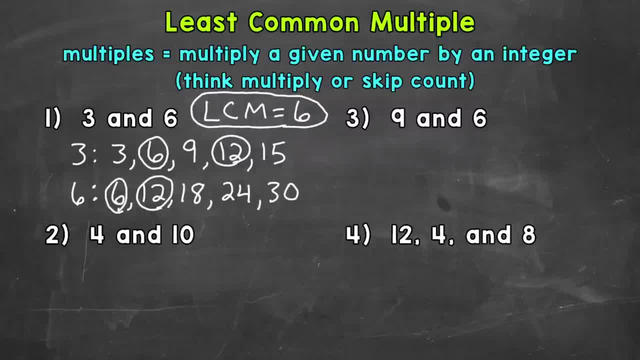 Let's try another example and move on to number two, where we have four and ten. So we'll start with some multiples of four. So skip count or think of it as four times one, four times two, so on and so forth. Let's skip count for this one. 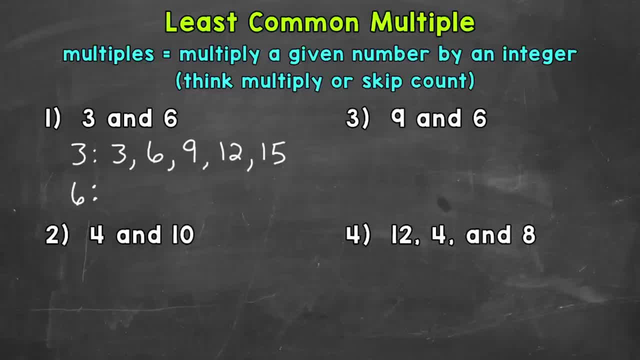 So again, think, multiply or skip count. So six times one is six, Six times two is twelve, Times three is eighteen, Times four is twenty-four, And then times five is thirty. So we did five multiples for each. Let's see if we have any common multiples. 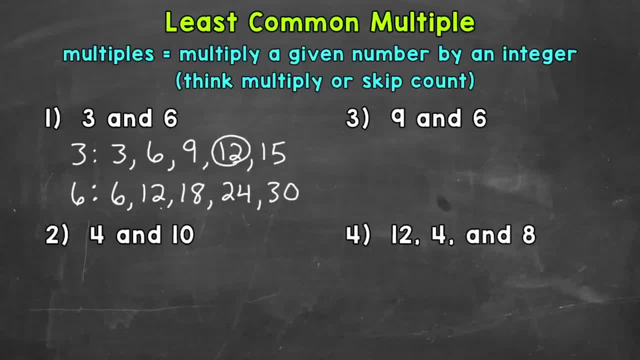 So we have twelve in common And we also have six in common, But we want the least. So six is going to be the least. It's going to be the least common multiple between three and six. So I'll put LCM, which stands for least common multiple, equals six. 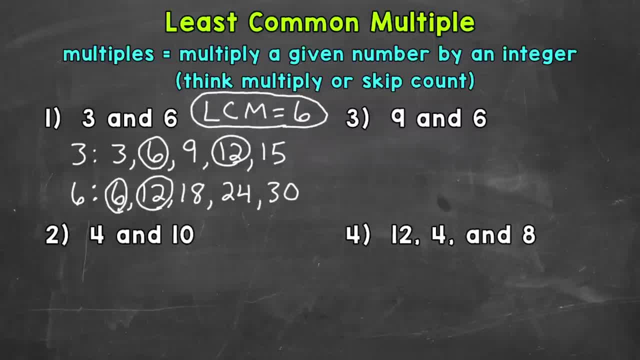 Let's try another example and move on to number two, where we have four and ten. So we'll start with some multiples of four. So skip count or think of it as four times one, four times two, so on and so forth. Let's skip count for this one. 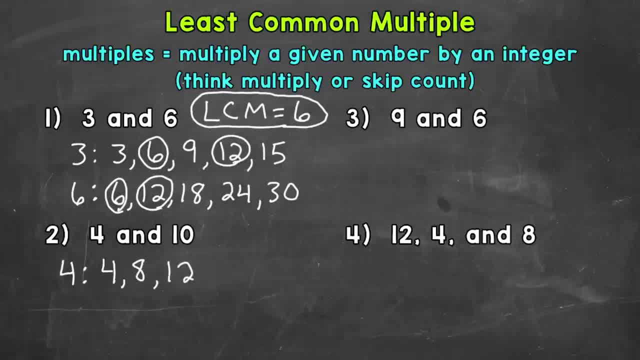 Four, eight, twelve, sixteen, twenty. So we'll write five for that one. Let's do ten now, Ten, twenty, and you may notice that we have something in common there, And that's going to be the least common multiple. 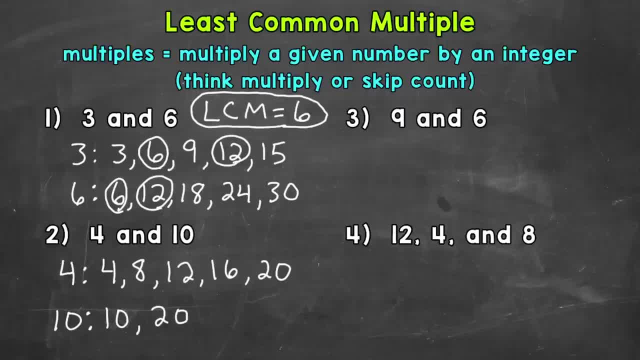 If you notice that you have a least common multiple, there's no need to keep writing out multiples. We have our answer. So twenty is going to be our least common multiple. So least common multiple equals twenty. Let's move on to number three, where we have nine and six. 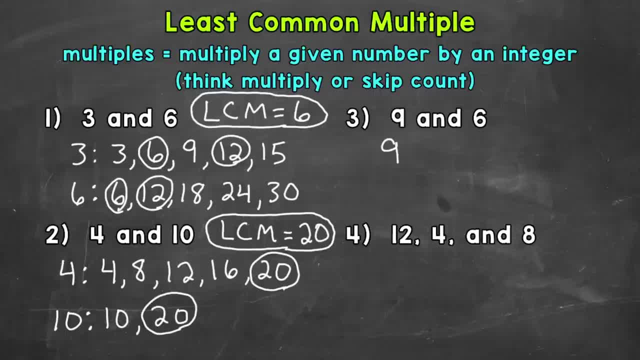 So we'll start with some multiples of nine here, So nine, eighteen, twenty, Eighteen, twenty-seven, thirty-six, forty-five, And now some multiples of six, Six, twelve, eighteen, And we have our least common multiple right here, which is going to be eighteen. 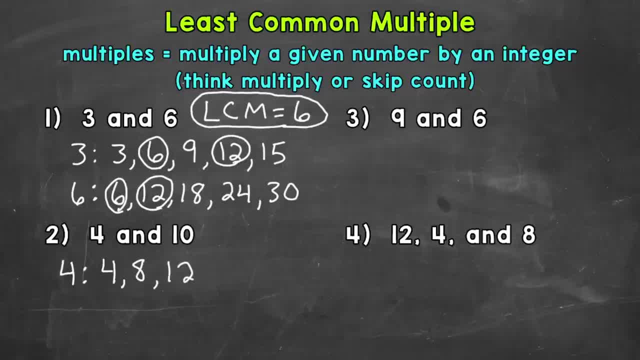 Four, eight, twelve, sixteen, twenty. So we'll write five for that one. Let's do ten now, Ten, twenty, And you may notice that we have something in common there, And that's going to be the least common multiple. 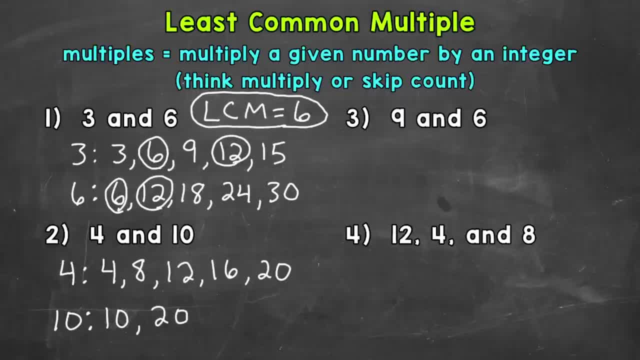 If you notice that you have a least common multiple, there's no need to keep writing out multiples. We have our answer. So twenty is going to be our least common multiple. So least common multiple equals twenty. Let's move on to number three, where we have nine and six. 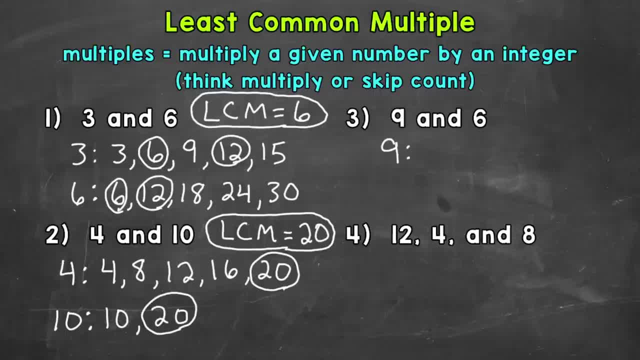 So we'll start with some multiples of nine here, So nine, eighteen, twenty-seven, Twenty-seven, thirty-six, forty-five, And now some multiples of six, Six, twelve, eighteen, And we have our least common multiple right here, which is going to be eighteen. 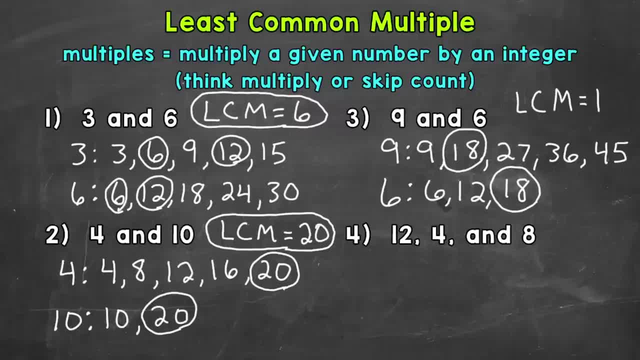 So our LCM equals eighteen. I do want to mention, before moving on to number four, that for these problems we're going to have an infinite amount of common multiples. Since we have an infinite amount of multiples, we're therefore going to have an infinite amount of common multiples. 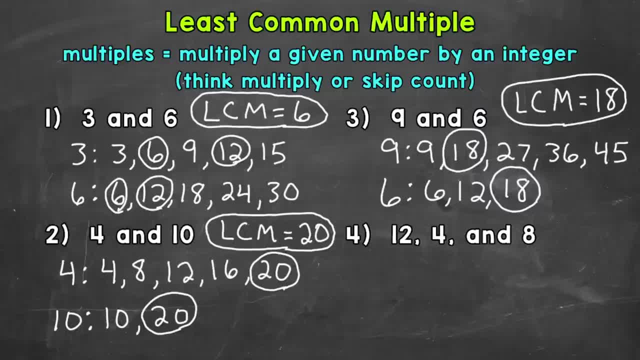 We can always extend our lists further in order to find more common multiples, But since we want the least, we need to focus on that least, And once we have that least common multiple, we have our answer. Let's move on to number four, where we have twelve, four and eight. 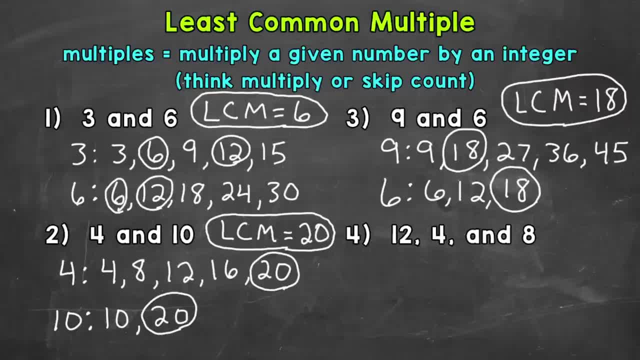 So we have three numbers and we need to find the least common multiple between all three. Let's start with some multiples of twelve, So twelve, twenty-four, thirty-six, forty-eight and sixty. Let's do four now, So four, eight, twelve, sixteen and twenty. 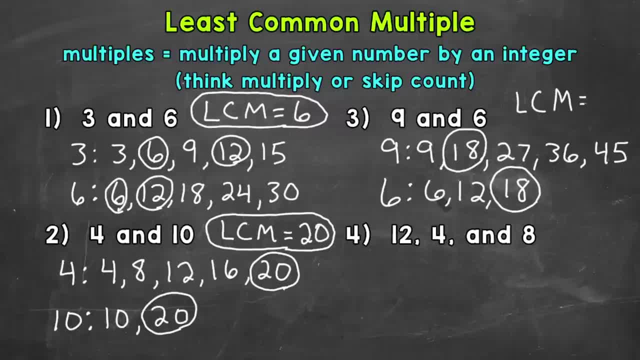 So our LCM equals eighteen. Now I do want to mention, before moving on to number four, that for these problems we're going to have an infinite amount of common multiples. Since we have an infinite amount of multiples, we're therefore going to have an infinite amount of common multiples. 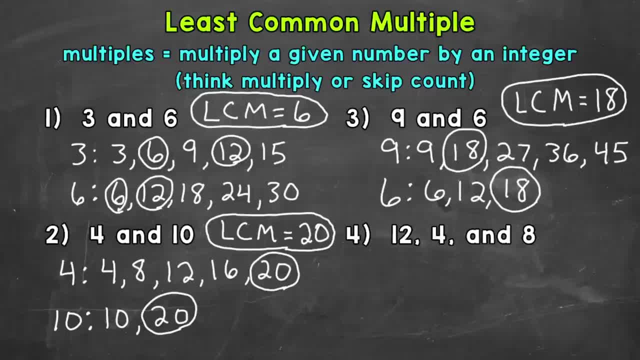 We can always extend our lists further in order to find more common multiples, But since we want the least, we need to focus on that least, And once we have that least common multiple, we have our answer. Let's move on to number four, where we have twelve, four and eight. 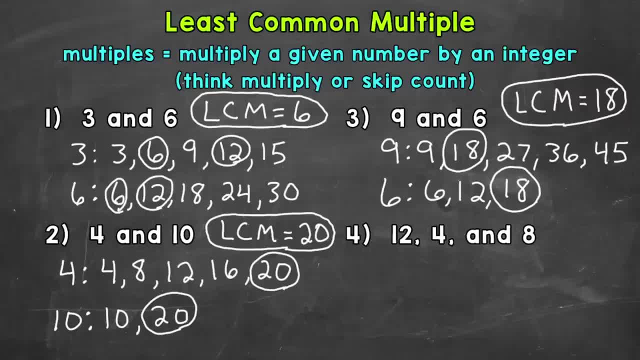 So we have three numbers and we need to find the least common multiple between all three. Let's start with some multiples of twelve. So twelve, twenty-four, thirty-six, forty-eight and sixty. So twelve, twenty-four, thirty-six, forty-eight and sixty. 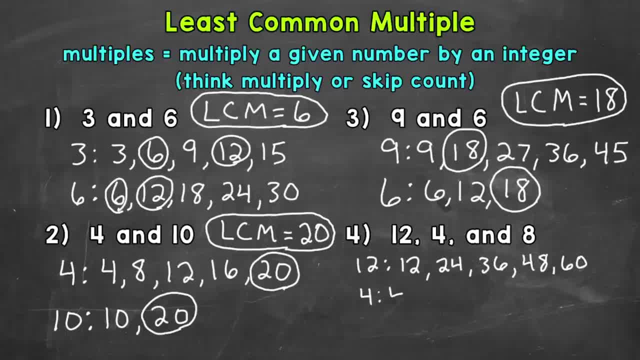 Let's do four now, So four, eight, twelve, sixteen and twenty, And lastly eight, So eight, sixteen, twenty-four, thirty-two and forty. So as we look at these lists, we do have some common multiples. 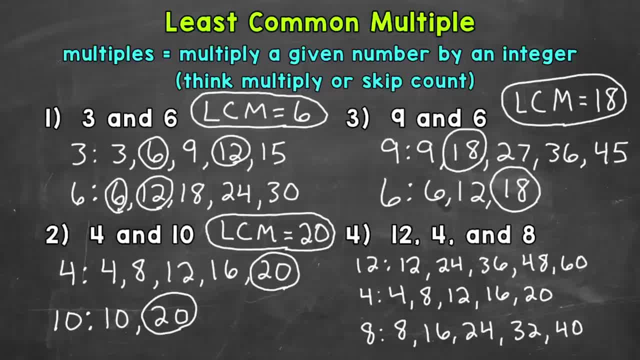 but we don't have any common multiples between all three And we need a common multiple between all three And specifically the least common multiple. So what we can do, we can extend our lists until we find that least common multiple. Now the twelves: 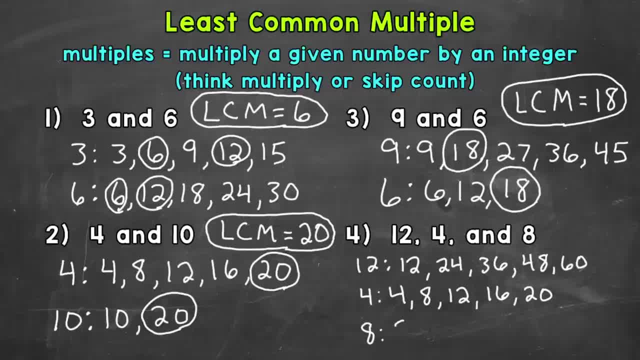 And lastly eight. So eight, sixteen, twenty-four, thirty-two and forty. So, as we look at these lists, we do have some common multiples, But we don't have any common multiples between all three, And we need a common multiple between all three. 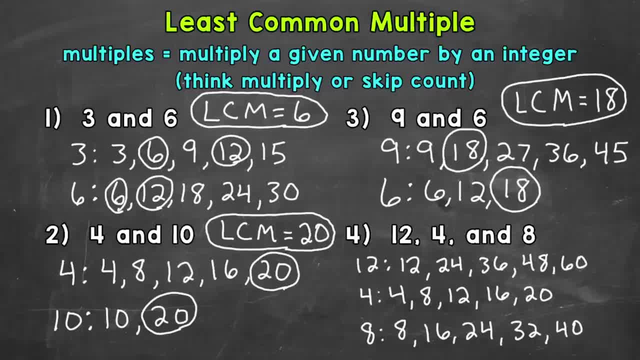 And specifically the least common multiple. So what we can do, we can extend our lists until we find that least common multiple, Now the twelves, the multiples of twelve. we're already at sixty, So let's leave that list. Let's look at the four. 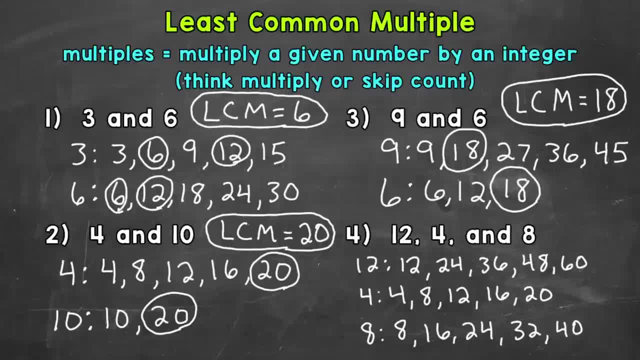 We're only at twenty there, So let's extend the lists of multiples for four. So our next multiple is going to be twenty-four And that's going to be our least common multiple: Twenty-four, twenty-four and twenty-four. So if you don't see a least common multiple, you can always extend your lists until you find it. 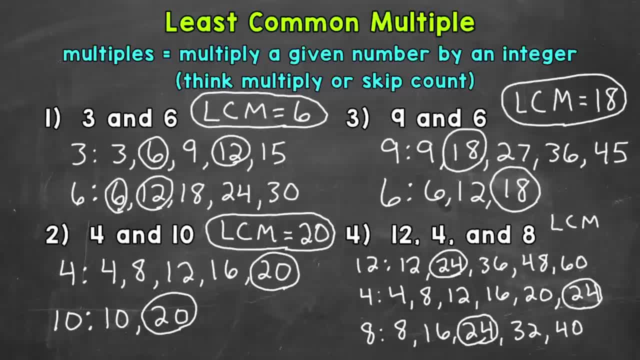 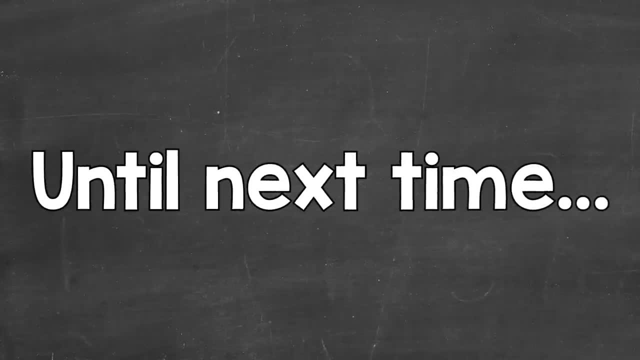 So for number four, our LCM equals twenty-four. So there you have it. There's how you find the least common multiple. I hope that helped. Thanks so much for watching. Until next time, peace. 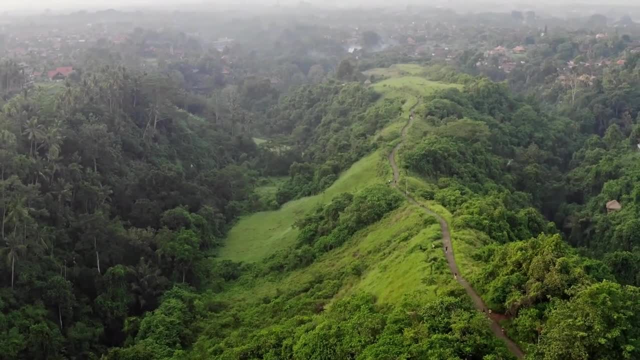 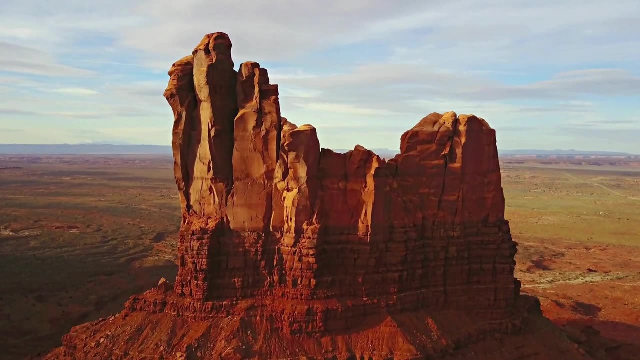 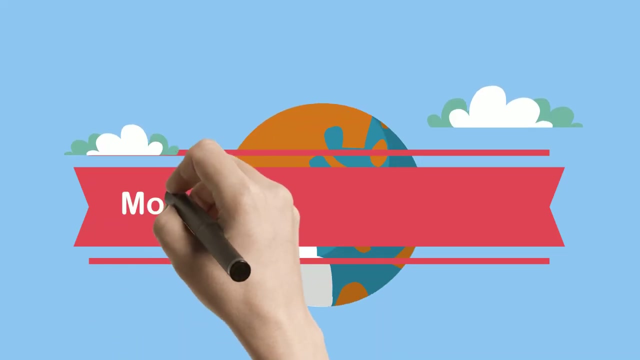 A typical rainforest can support thousands of trees of the same species. A desert may not be able to support a single tree. Each of these environments have different amounts of resources like food, water and shelter, and this impacts the population size. Welcome to MooMooMath. and Science and factors that affect population size. 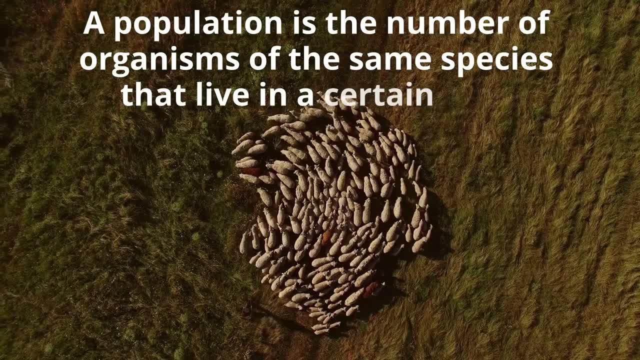 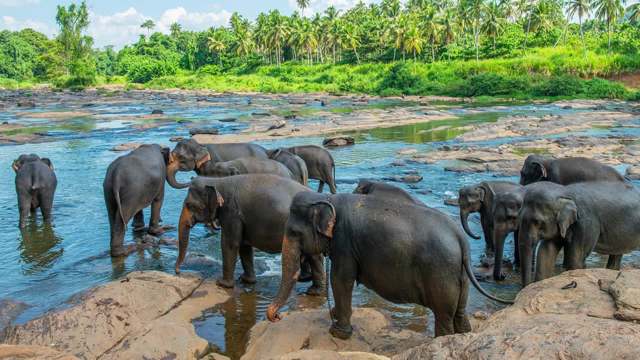 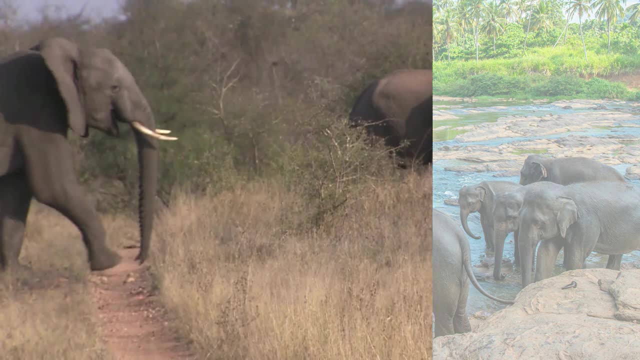 A population is the number of organisms of the same species that live in a certain area. For example, you can have a population of elephants. If the resources are plentiful, like food, water, shelter, then the population may grow. If the resources are scarce, then the population may. 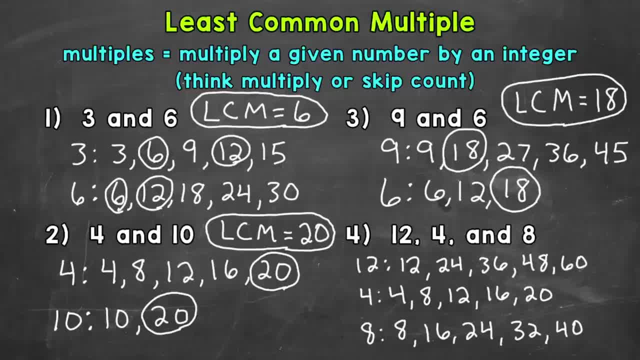 the multiples of twelve. we're already at sixty, So let's leave that list. Let's look at the four, So let's extend the lists of multiples for four. So our next multiple is going to be twenty-four, And that's going to be.